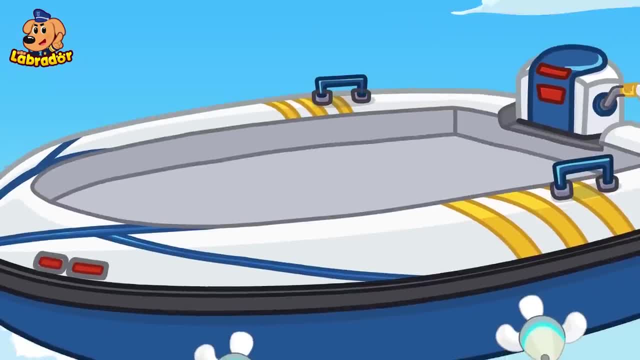 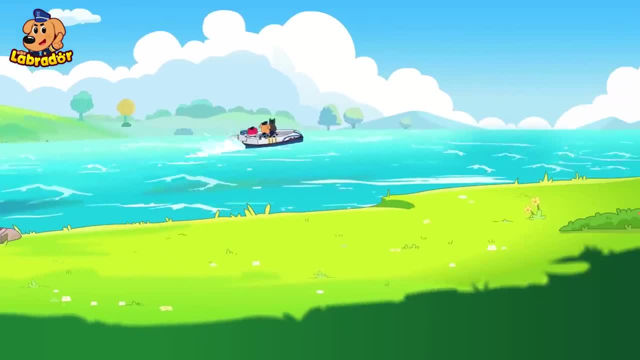 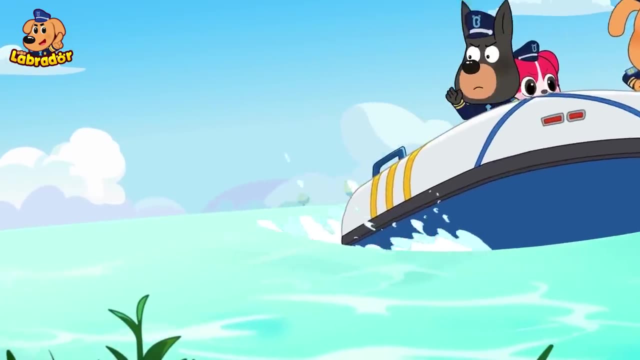 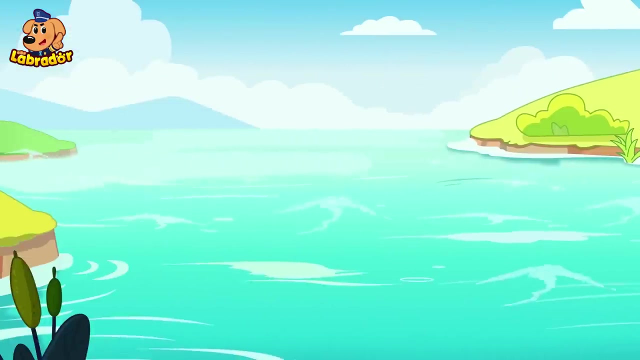 Papio always has a way. Super speedboat, Let's go. Please find my friends. Little elephant, Little rhino, Little rabbit, Little rabbit, Little rabbit. Little rhino, Little rhino, The water monster is real Thema. 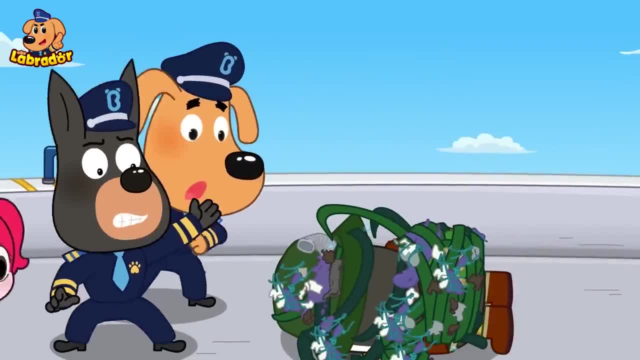 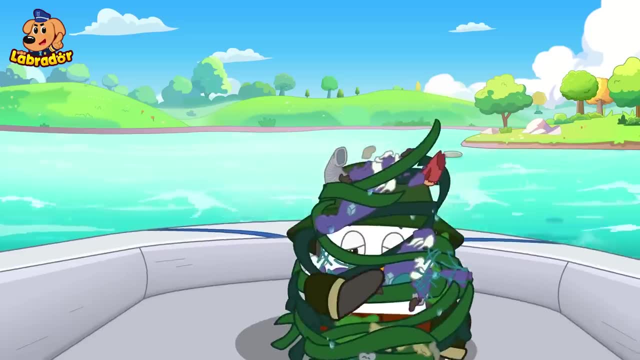 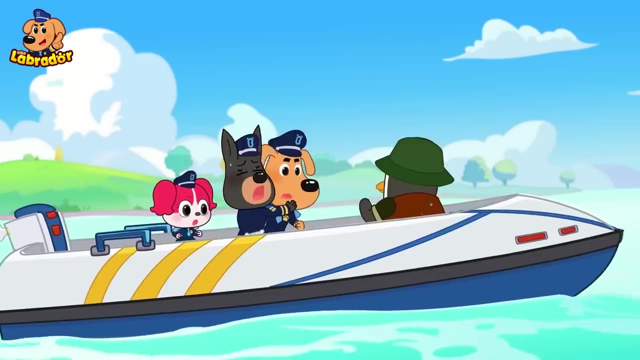 Oh, ah, Ah, Hi there M-m. Hi there, The water monster is real. Ow, I'm not a water monster, I'm Mr Pangolin. I'm Mr Pangolin Penguin. what happened to you? 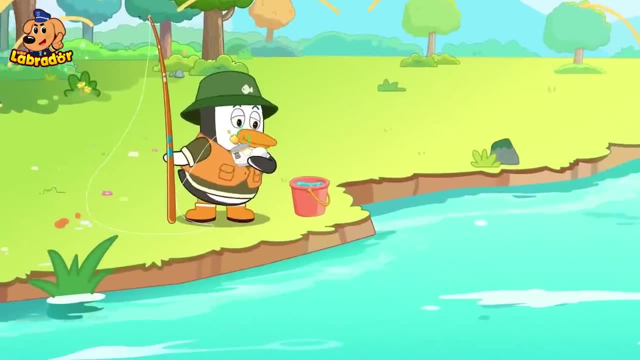 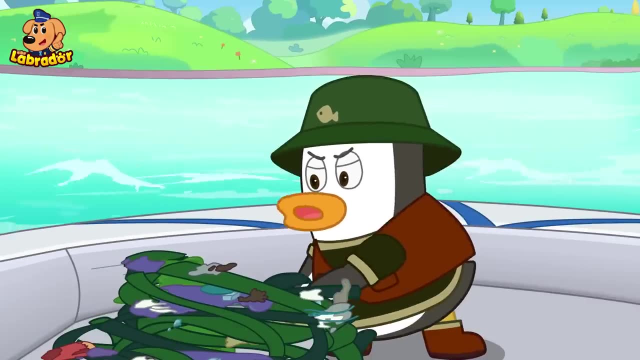 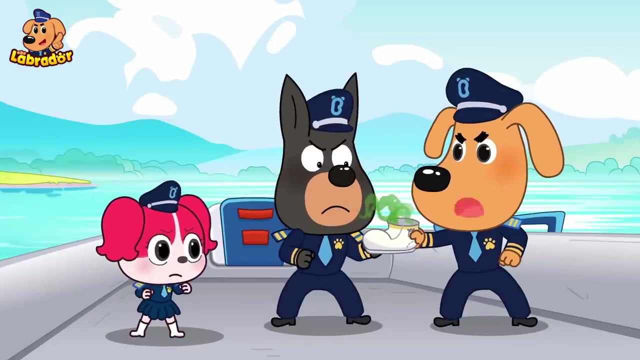 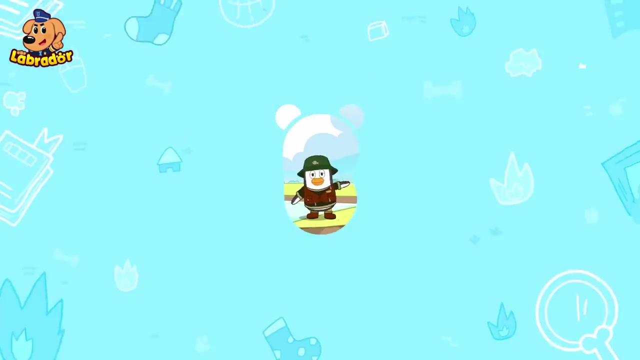 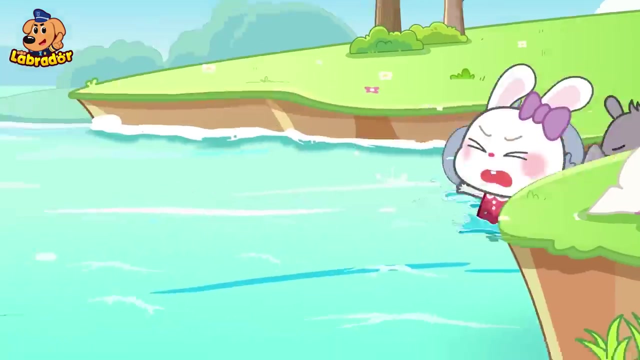 Oh my, I was fishing by the shore and caught a smelly shoe that nearly knocked me out. Thank you for saving me. This is the shoe. This is Little Rhino's shoe. This way, Good luck, Don't take us. Let us go. 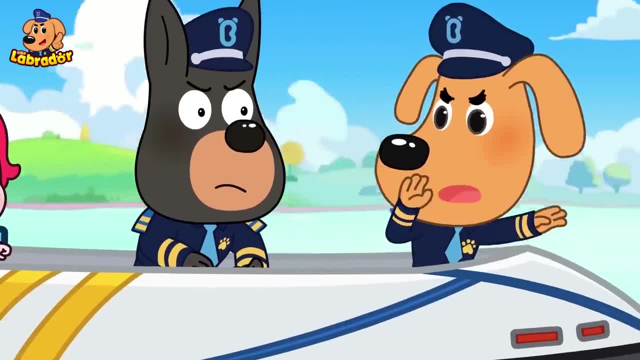 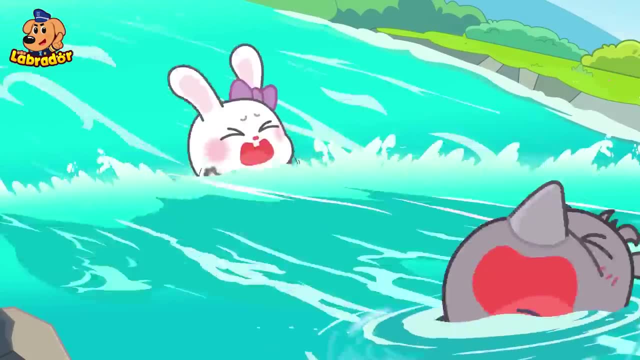 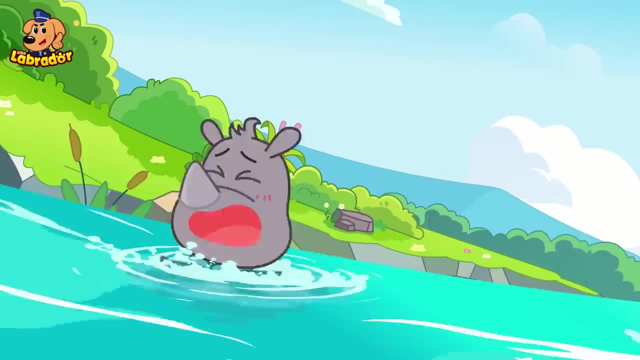 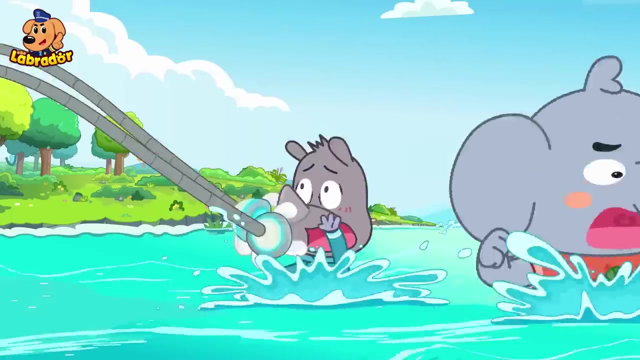 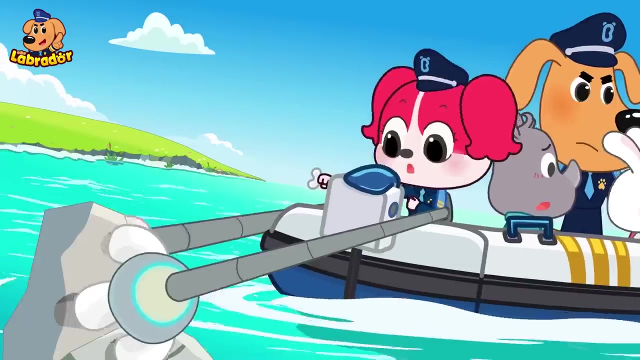 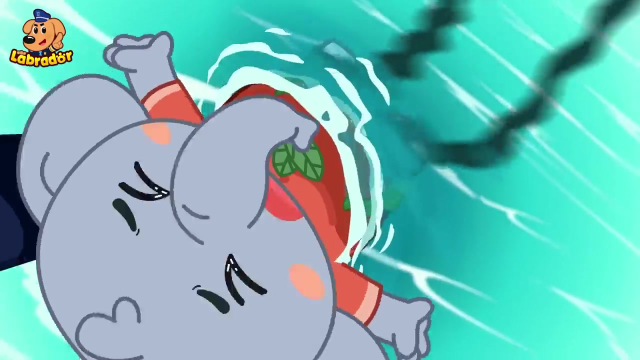 Look Over there, Papillon speed up, Got it. Help us. Help, Don't worry, We'll save you. Help, Watch out, Watch me. I can't pull him up. The water monster's pulling me. It can't be. I'll go check it out. 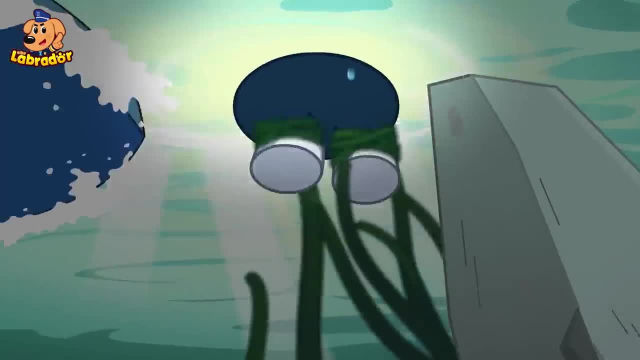 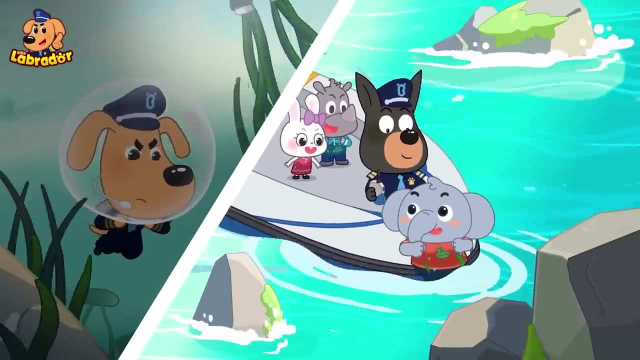 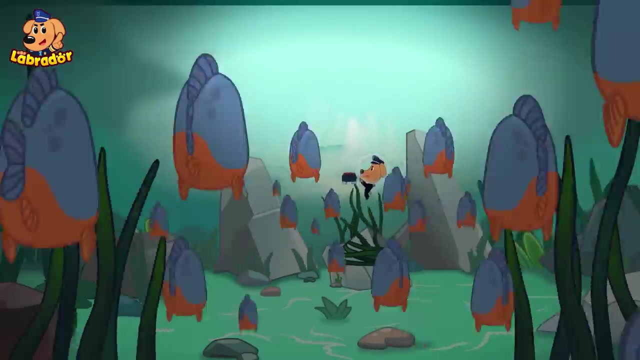 I'll go check it out. The water monster is just water playing. Phew, That's what it was. Oh no, I need to hurry. You're safe now Run. Piranhas are coming. Piranhas are coming.